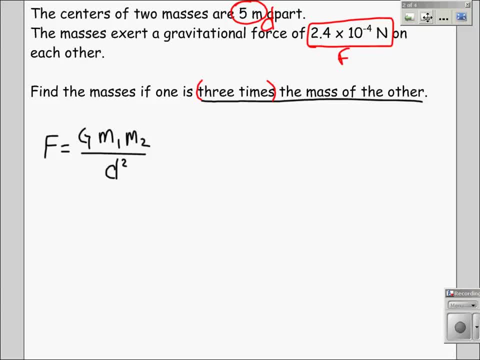 Now how I like to proceed here is to give these masses a name: Mass 1 and mass 2.. Now, what is mass 1 equal to? Well, let's just call it m. And if mass 1 is m and mass 2 is 3 times the size of mass 1, then we'll call it 3m. 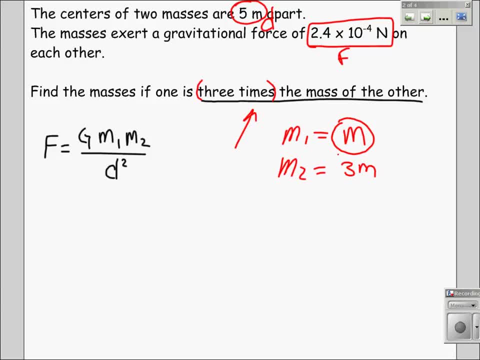 So we have the name. So we have the names now of our masses: Mass 1, we'll call m. Mass 2, we'll call 3m. Going back to our equation, let's go ahead and fill those values in: F equals universal gravitational constant times m, times 3m. 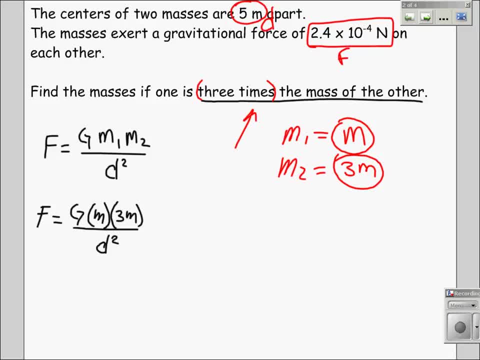 Those are the names of those Divided by d squared. Now I'm going to go ahead and manipulate this equation to get m by itself first, before I plug in the numbers. It just goes quicker that way You're not having to write the numbers over it again. 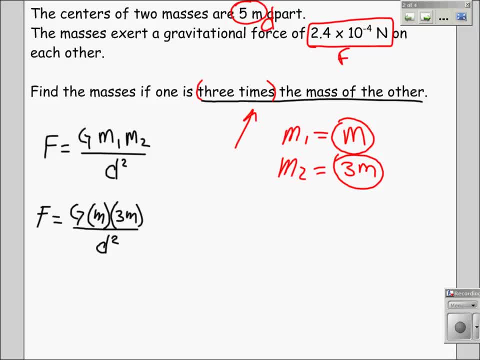 You could plug the numbers in now and then manipulate the equation. I just find it easier to do it this way. So let's simplify this by taking out the parentheses, because it doesn't matter the order in which we multiply those four items. 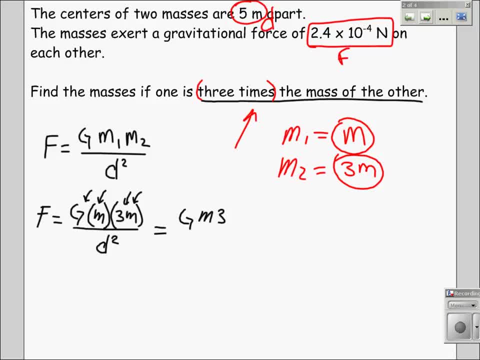 So we'll say that g times m times 3 times m over d squared. And we can simplify that one more time In saying, in rearranging, g3 times m squared divided by d squared. So here's our equation that we're starting with then. 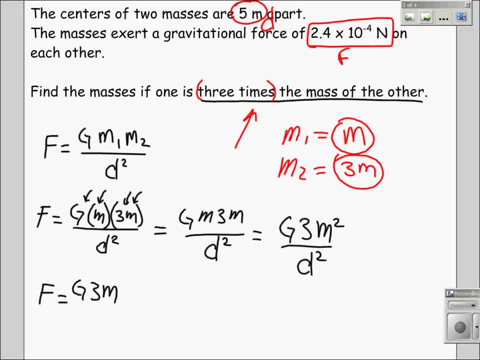 F equals g3m squared over d squared, And we need to get m by itself. So the first thing we should do is multiply. Let me see if I can get this. Give us some more room to work with here. We'll just copy that and move it to another page. 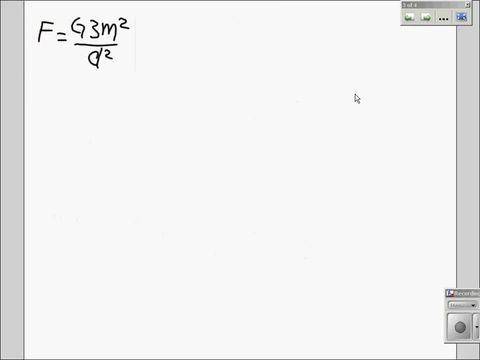 How about that? Give us plenty of room to work, All right. And we can say here that multiply both sides by d squared, So f times d squared equals g3m squared, And then divide both sides by g3. So 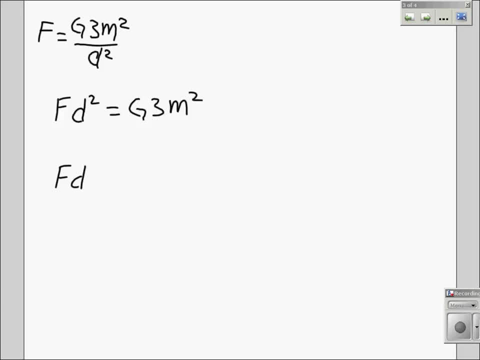 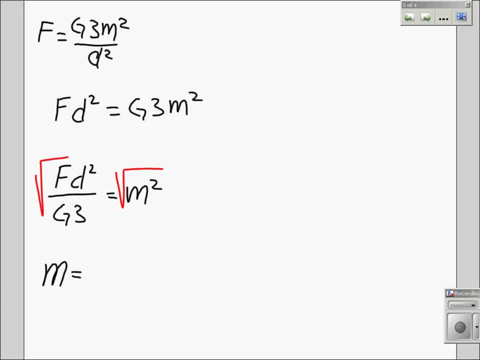 Well, if that's true, then m is equal to the square root of f times d, squared divided by g times 3.. And let's do this one more time, So we'll copy that, excuse me, and move it to there. 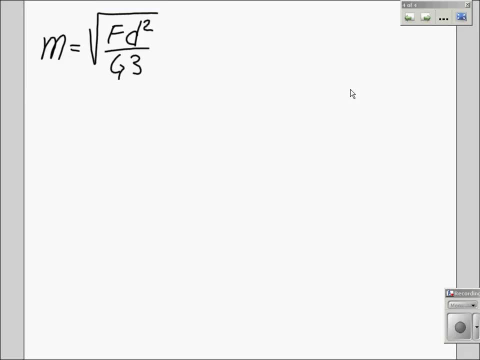 Give us plenty of space to work now. So the the values that we have. going back and looking at that, sorry. the mass is equal to the force, which we said was 2.4 times 10 to negative 4 newtons. 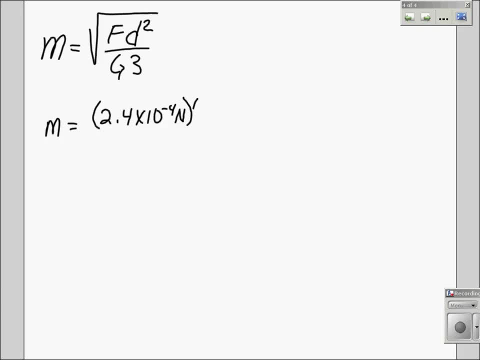 So so times the distance squared in this case was 5 meters, so that's 25 meters squared. We're dividing that by g, which is 6.67 times 10, to the negative 11, and that's newtons times meters squared over kilograms squared. 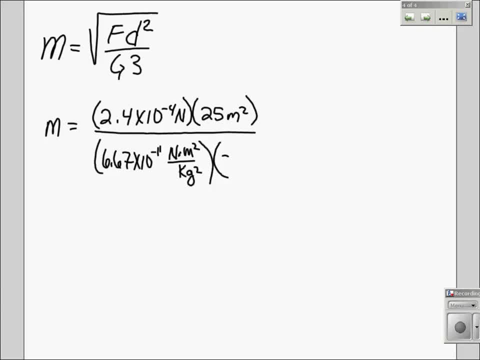 And we're multiplying that by 3, and it's the square root of that guy. So something that we should notice right away: newtons are going to cancel out, meters squared are going to cancel out, leaving us only with kilograms squared. 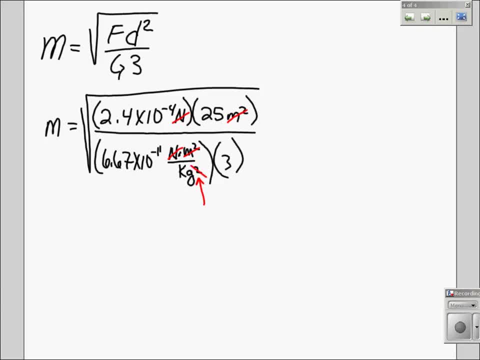 But that is going to go away too, because we're going to take the square root of those numbers. So if you take 2.4 times 10 to the negative, 4 times 25, and then divide that by this value, 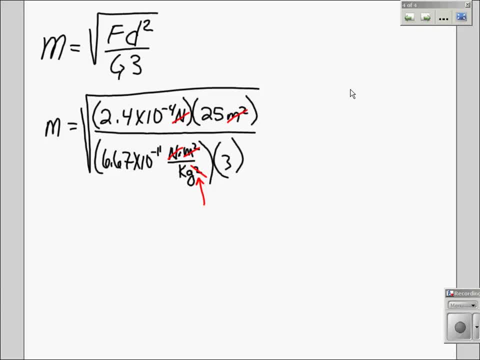 6.67 times 10 to the negative 11 times 3, take the square root of all that and you'll get a value of around 5,476 kilograms. So that's m, Therefore m1, we'll call 5,476 kilograms.